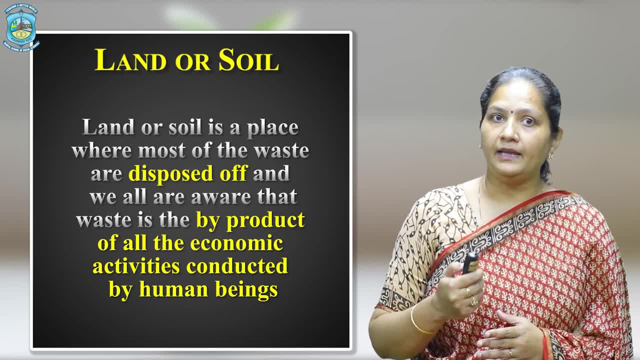 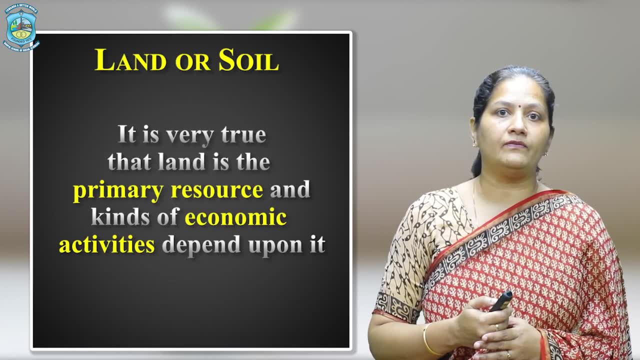 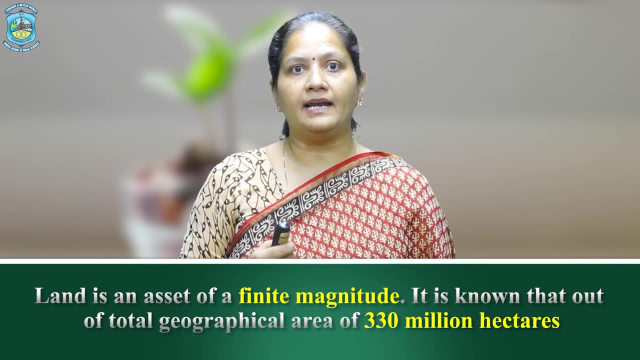 Soil provides us food, medicine, material for our survival. It is very true that land is the primary resource and all kinds of economic activities depend upon land resources. Land is an asset of a finite magnitude. It is known, and these are the lasers of man's body. Which usimizations are represented by muri water. it is known that out of total geological blocks, as well as of… New Lights elapses which will get through the days of hard work. The ball, A by A, is the gravity of winds, mud, of the bodies of sand or, here, the momentum of the earth, soil, of land and water. 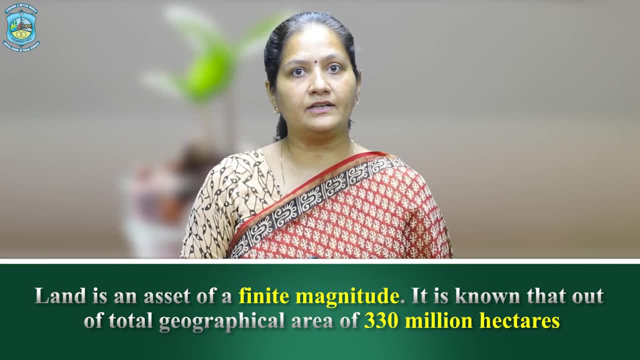 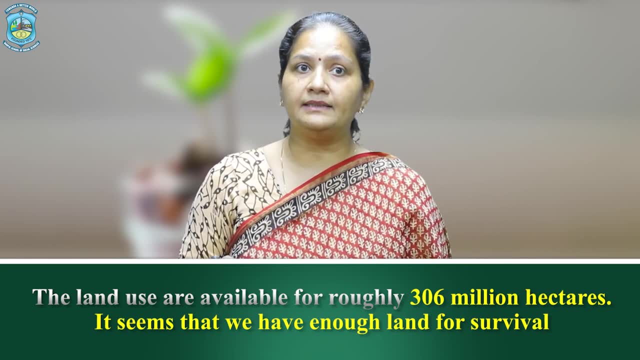 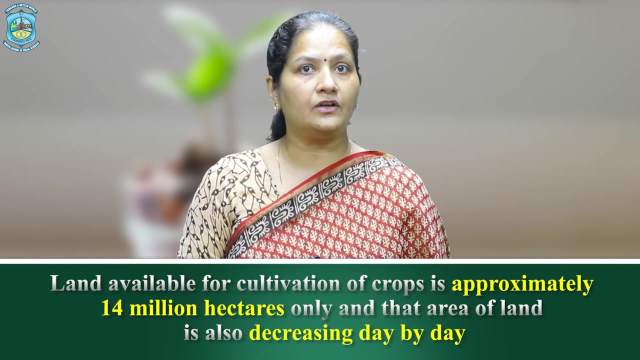 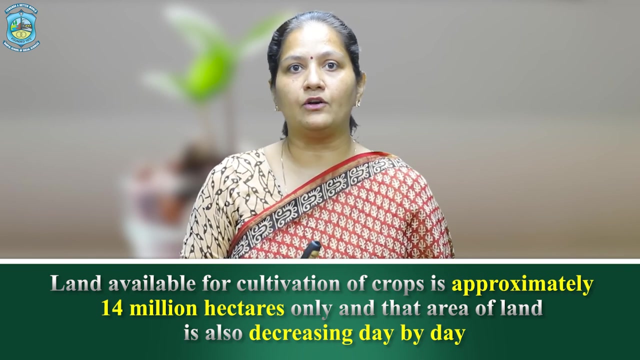 total geographical area of 330 million hectares. the land use are available for roughly 306 million hectares. It seems that we have enough land to use, but we do, though we do, but the land available for cultivation of crop is approximately 14 million hectares only, and that area of land is 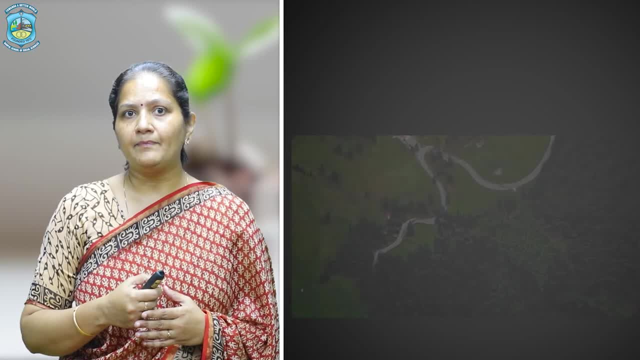 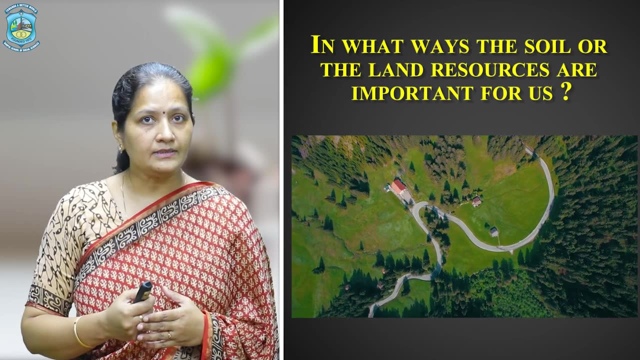 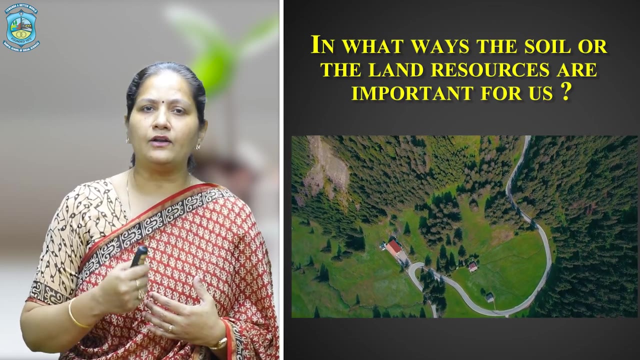 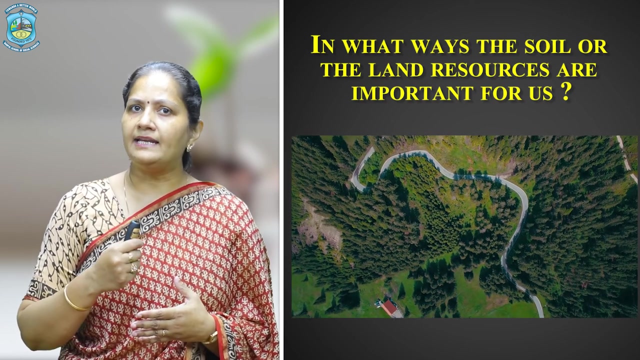 also decreasing day by day. Let us see what ways the soil or the land resources are important for us. Land is the natural resource that support natural vegetation, wildlife, economic activities, transport and all the communication system. We grow our food and energy on land: 95% of our food. 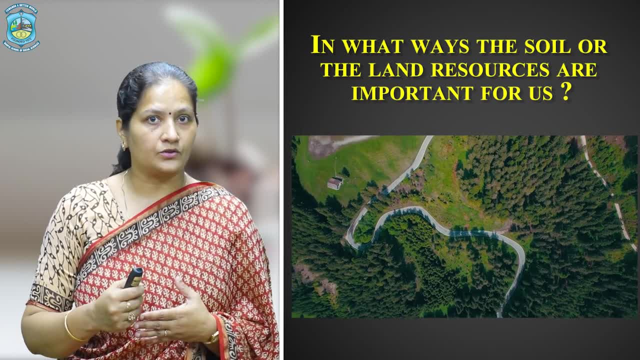 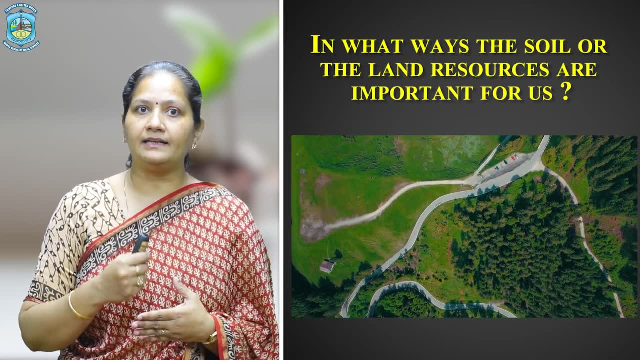 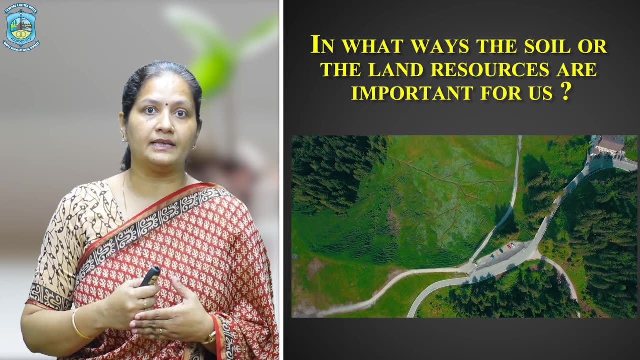 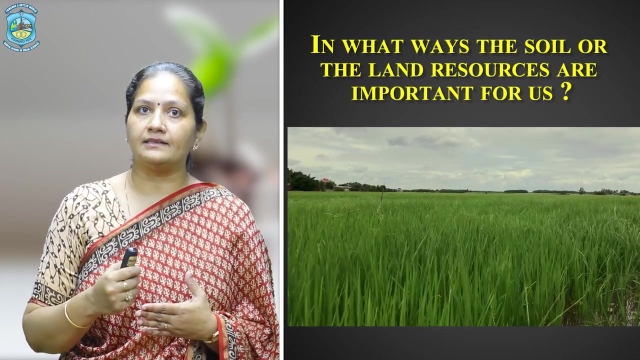 comes directly or indirectly from soil. On land all the economic activities are performed. We can say that land is the foundation of economic growth, but we always take land and land resources for granted. We human beings degrade the land and that is the life-giving asset. Every year, we lose approximately 24 billion tons of the fertile soil. 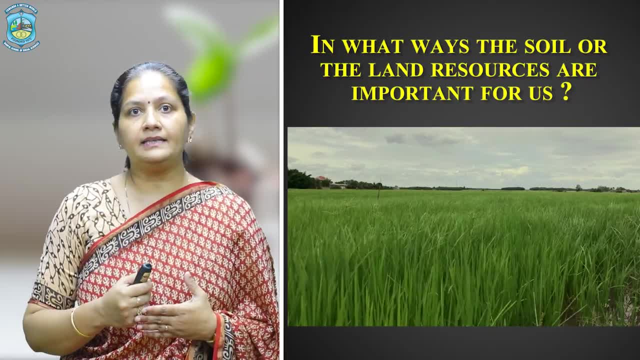 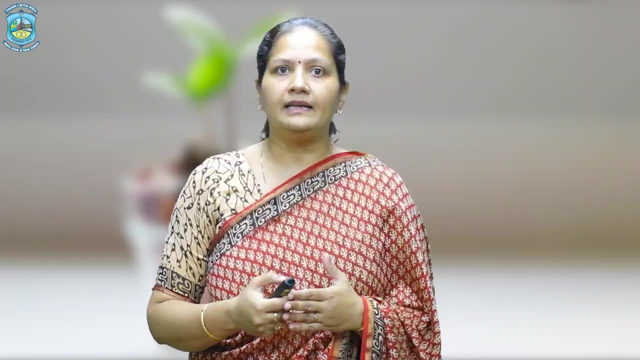 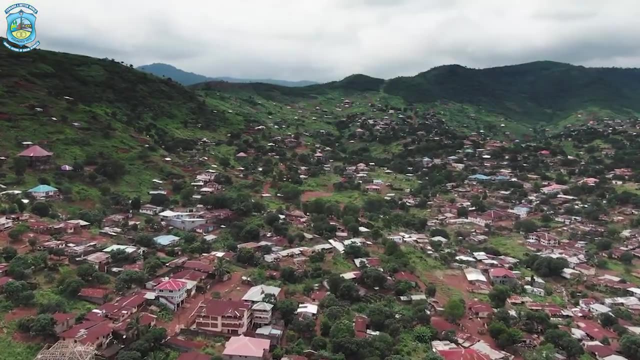 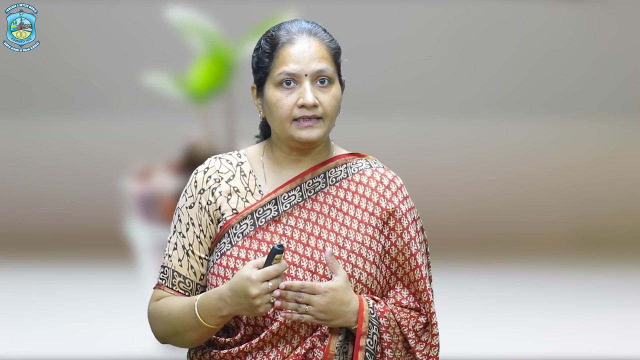 due to degradation. These are all the entities that cover some of our fertile and productive land as well. So it is very clear that we are dependent on land for our food, for our habits, for transport and what not. But, dear students, this land, or soil resource, is continuously degraded. That land degradation is now a global 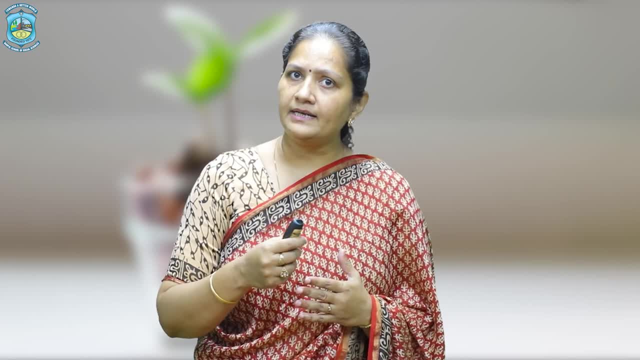 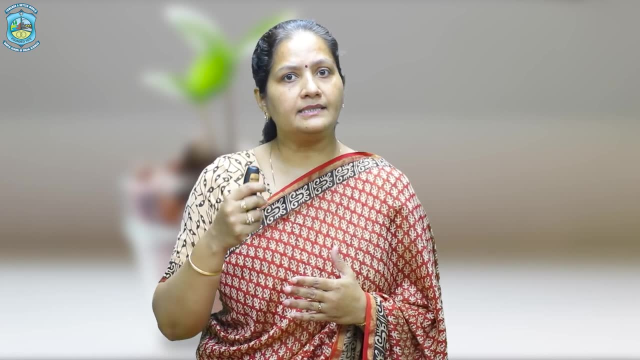 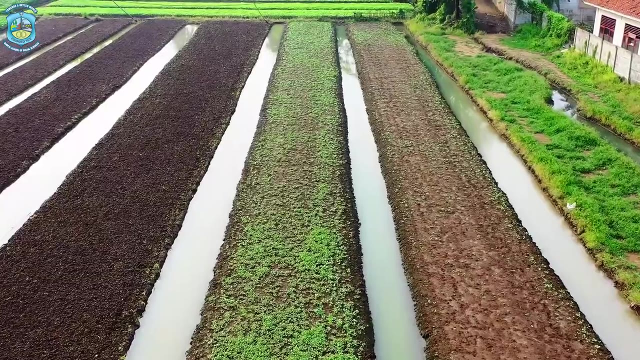 problem. This land degradation is both quantitative and qualitative in nature. It means that the air area of the land is degrading and, at the same time, the fertility or the quality of land or soil is also degrading. There are various causes of this land degradation. 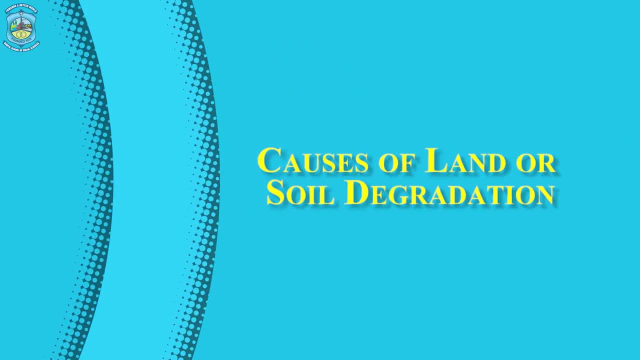 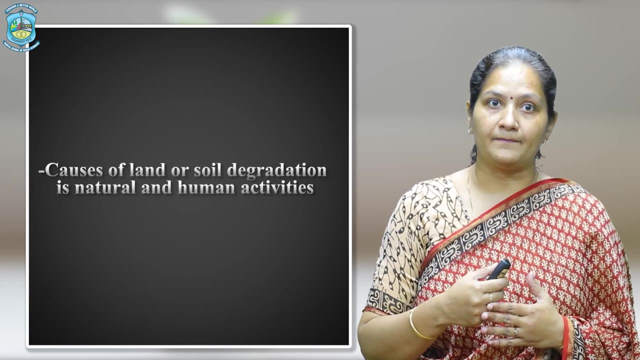 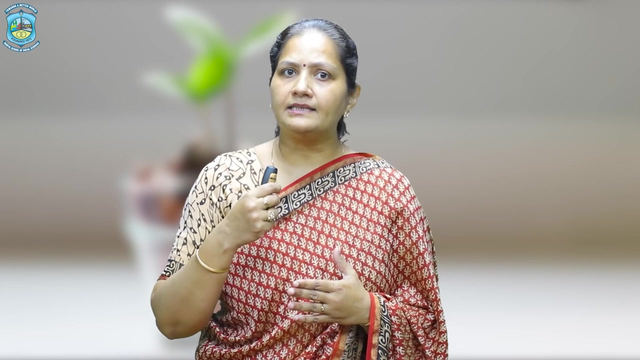 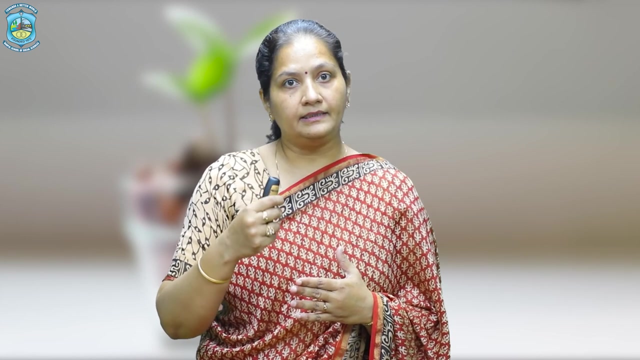 Now let us discuss the causes of land or soil degradation. The causes of land degradation is natural and human activities as well. It means that some natural causes are contributing in the land degradation and, at the same time, some of the human actions are also accelerating the process of land degradation. The natural causes of land degradation are heavy rainfall. 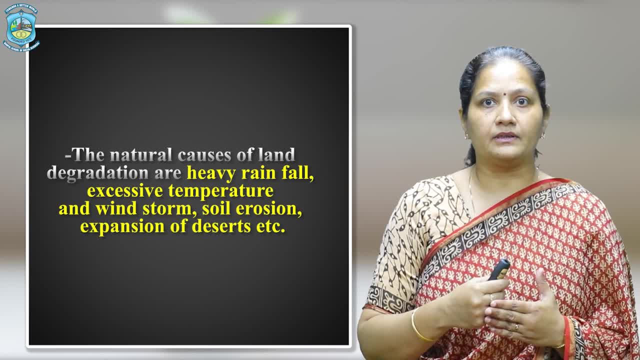 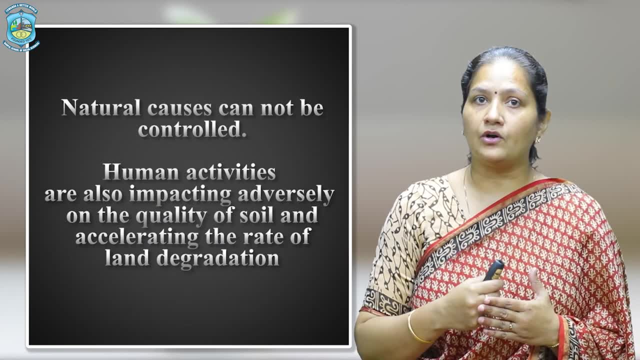 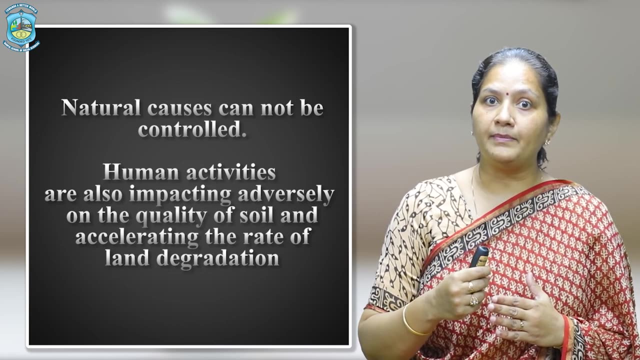 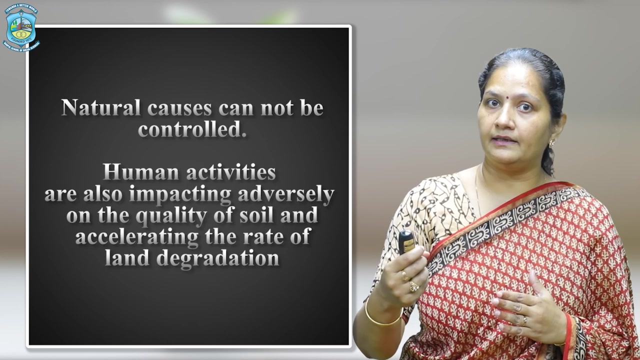 excessive temperature and windstorm, soil erosion, expansion of deserts, so on and so forth, and we all know that the natural causes cannot be controlled. A part of natural causes, human activities are also impacting adversely on the quality of soil and accelerating the rate of land degradation. When we talk about examples of human activities, there are so many. 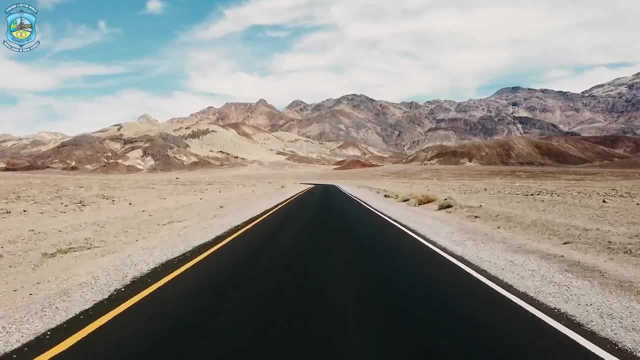 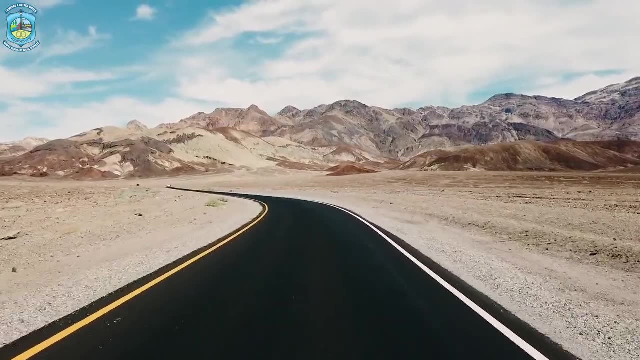 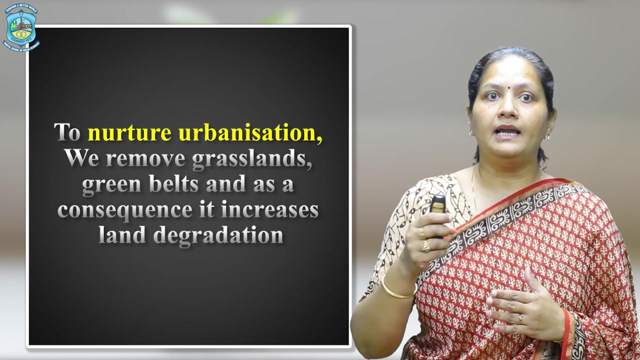 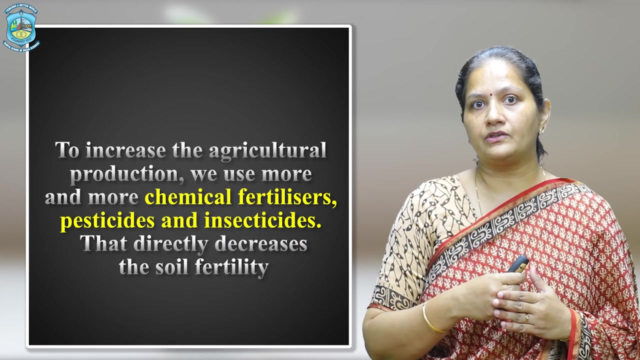 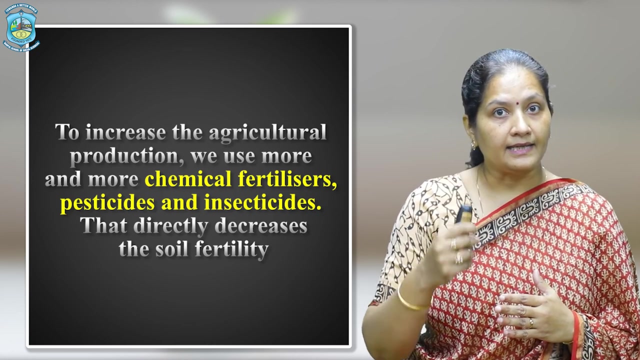 examples. We human beings are constructing roads for the sake of development, and that construction of road is increasing the rate of land degradation. To nurture urbanization, we remove grasslands, green belts and, as a consequence, it increases land degradation. To increase agricultural production, we use more and more chemical fertilizers, pesticides and insecticides. that directly 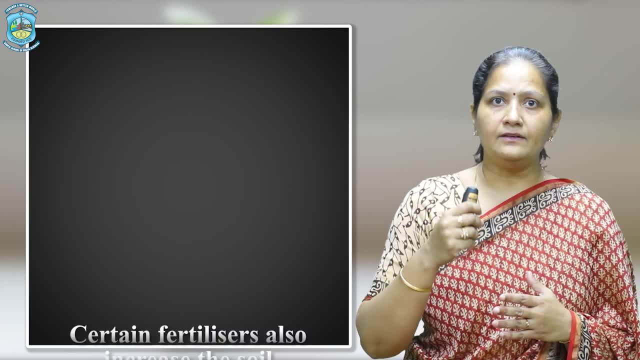 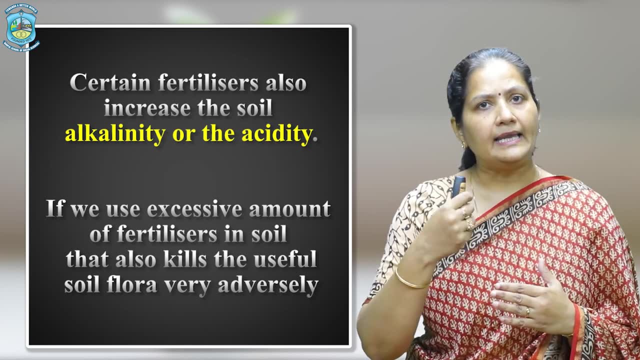 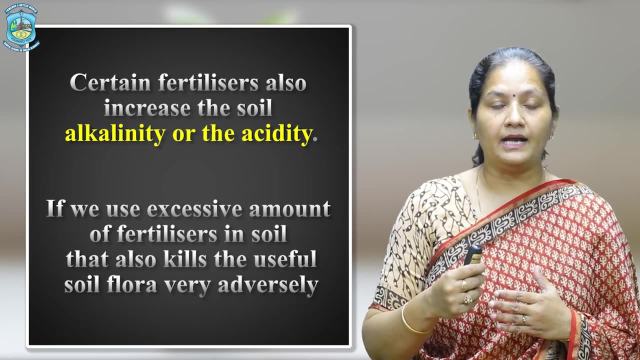 decreases the soil fertility. Certain fertilizers also increase the rate of land degradation To increase the soil alkalinity and acidity. If we use excessive amount of fertilizers in soil that also kills the useful soil flora very adversely. We human beings are very much in. 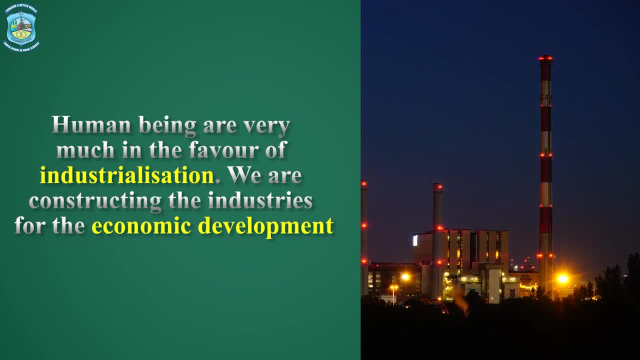 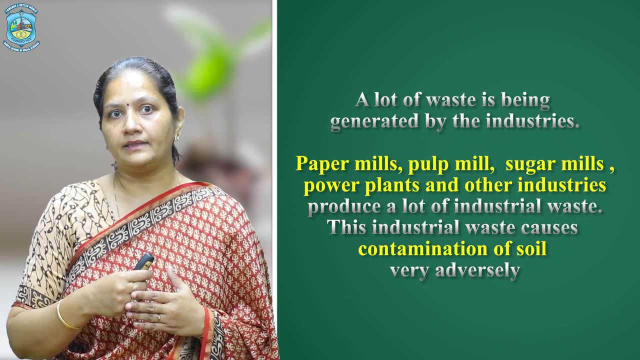 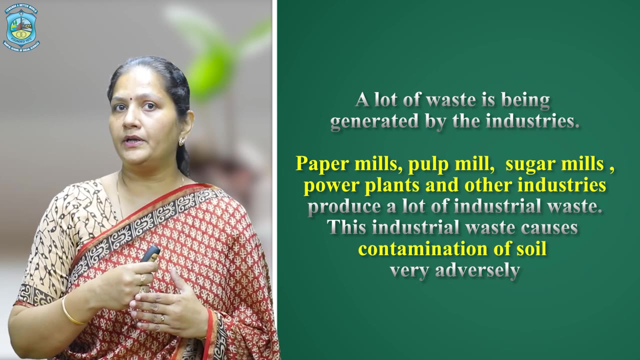 the favor of industrialization. We are constructing the industries for economic development. We all know a lot of waste is being generated by the industries. Paper mills, pulp mills, sugar mills, power plants and other industries also produce a lot of industrial waste. This industrial waste 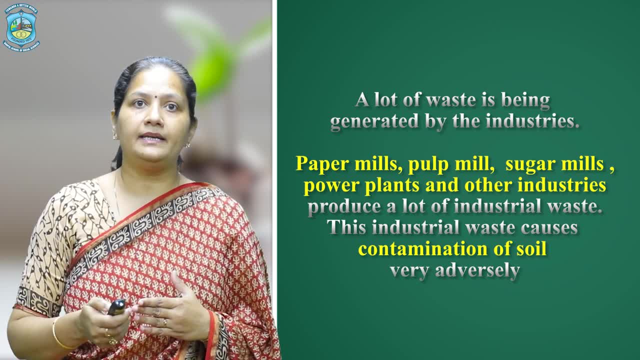 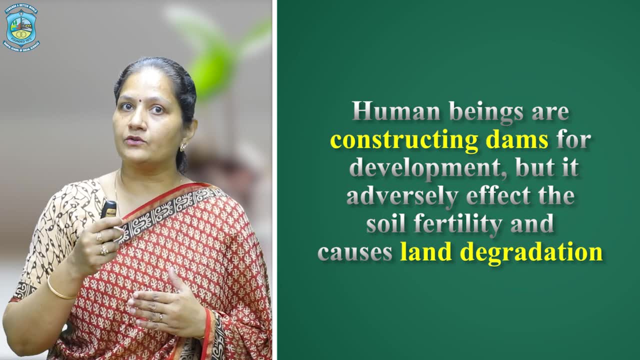 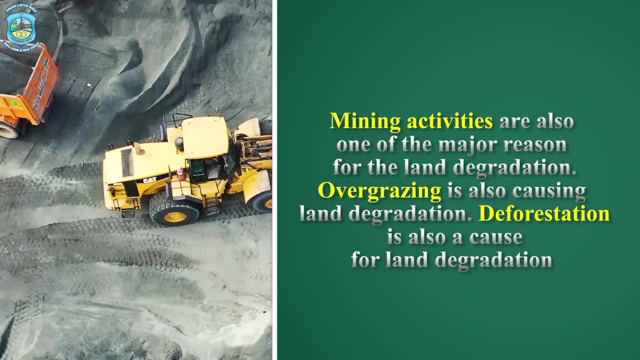 causes contamination of soil very adversely. We human beings are constructing dams for development but it adversely effect the soil fertility and causes land degradation. Mining activities are also one of the major reason for the land degradation. Overgrazing is also a very huge factor in the degradation and expand miteinander of the soil. In fact, overgrazing is a critical 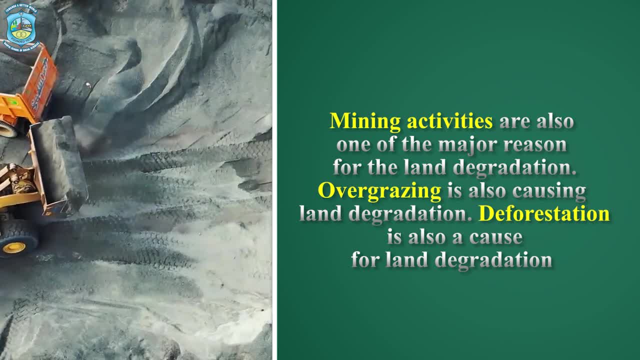 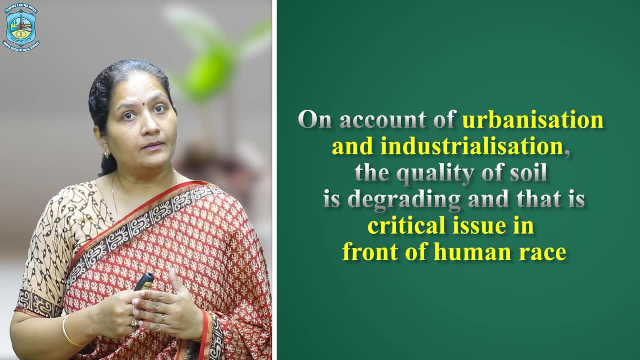 factor in the production of marinekład to smoketown Tunnel drainage and mininguper classy production, causing land degradation. Deforestation is also a cause for land degradation. We can conclude that on account of urbanization and industrialization, the quality of soil is. 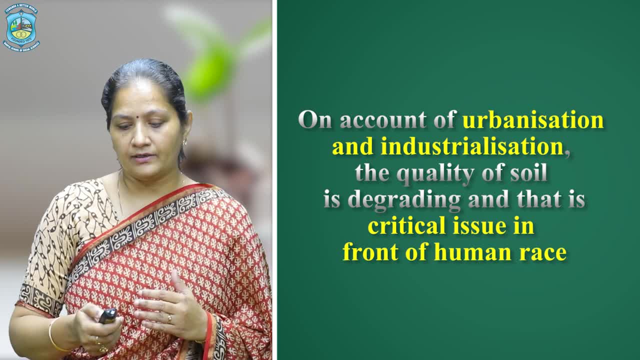 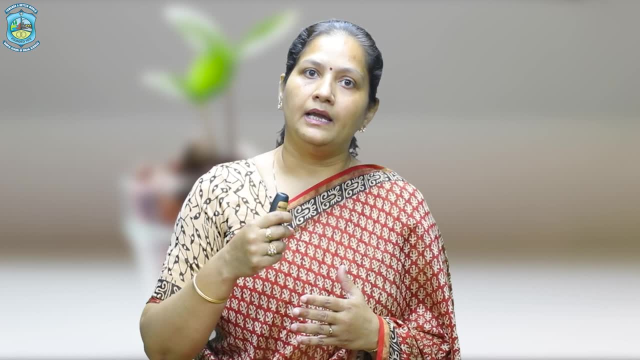 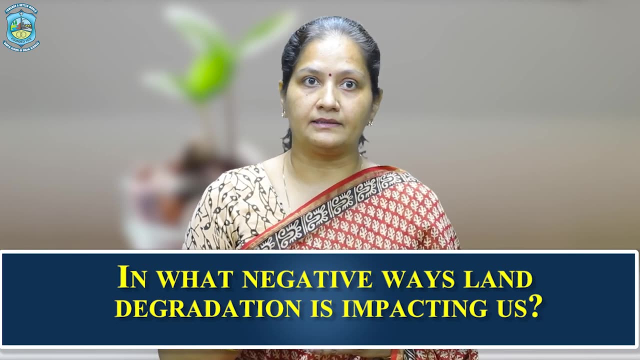 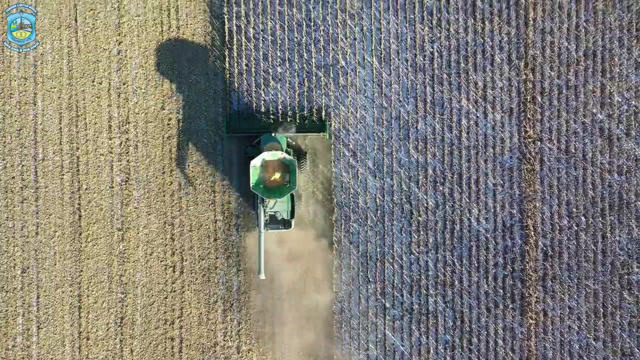 degrading, and that is very critical issue in front of human race. The land degradation is happening. it has a devastated impact on human life. Let us see in what negative ways land degradation is impacting us. Due to land degradation, there is a damage of topsoil. We should know that. if this 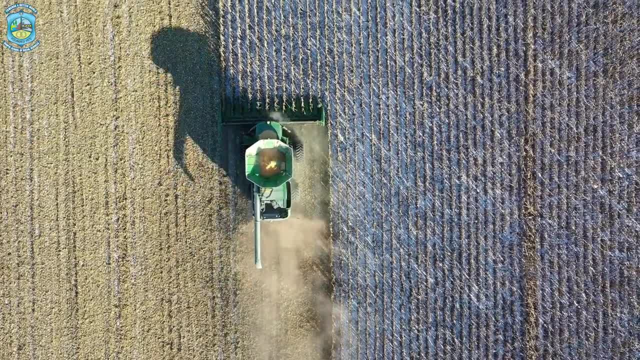 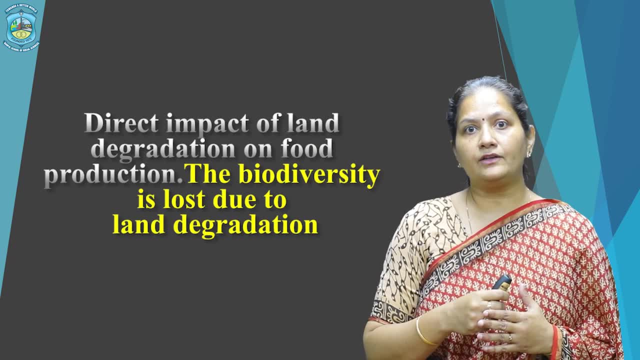 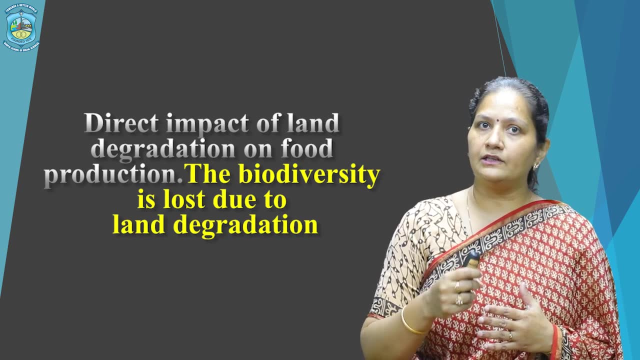 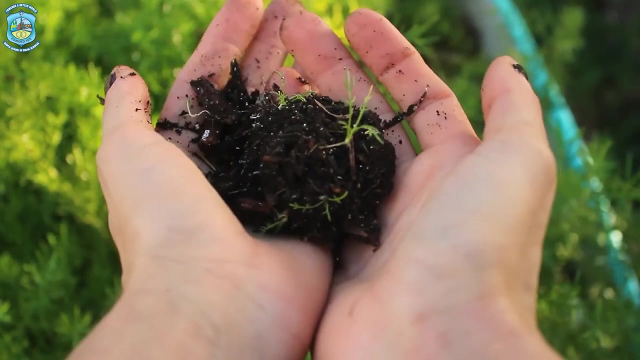 topsoil is damaged, the agricultural production will be reduced and that will lead to food scarcity. So there is a direct impact of land degradation on food. The biodiversity that is dependent on land is lost if there is land degradation. Land degradation leads to loss of soil fertility and loss of valuable nutrients Sometimes. 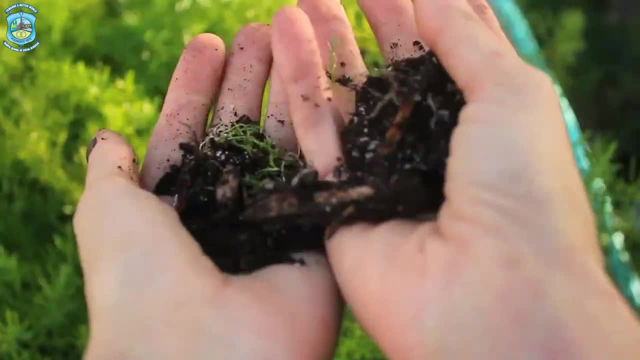 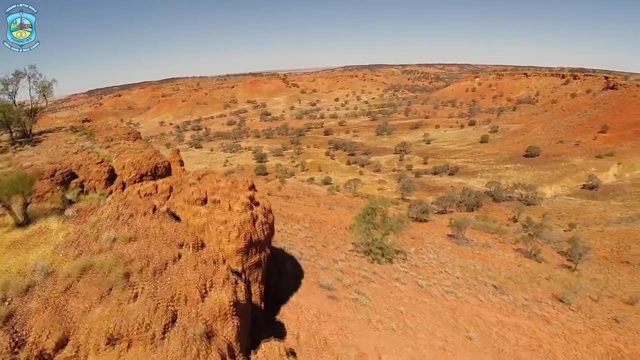 the land degradation leads to desertification. It means the fertile soil is converted into deserts. That is the worst condition of land degradation. So we can conclude that on account of urbanization, there is a damage of topsoil. We should know that. 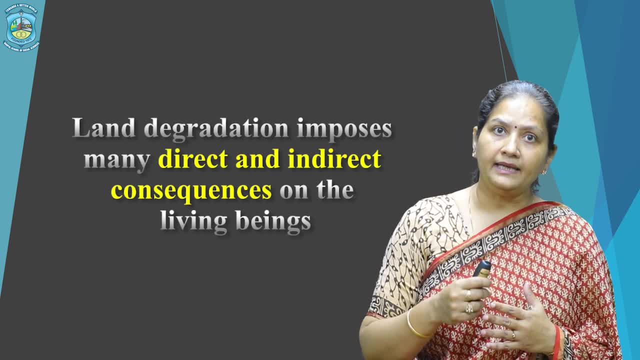 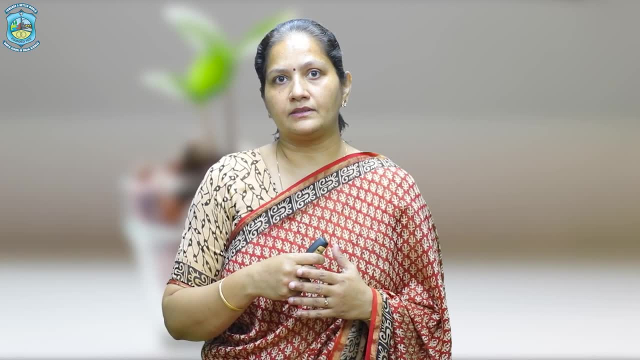 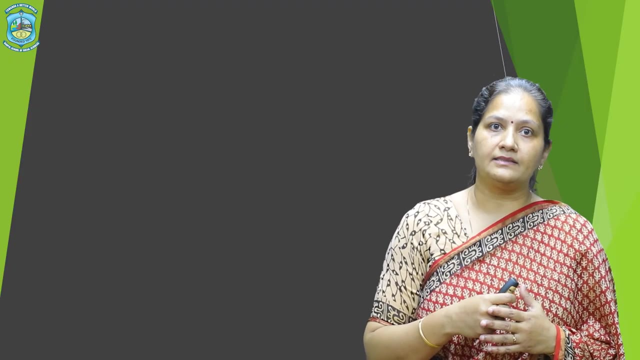 we can say that the land degradation imposes many direct and indirect consequences on the living beings. We have to conserve the land resources for the survival and for sustenance. This is our urgent need. So, how we can conserve the land, We have to find the measures of the conservation. 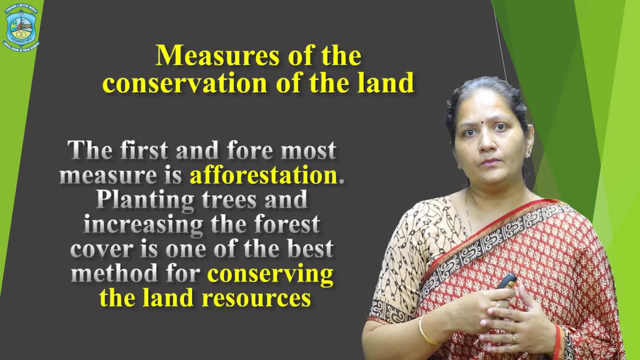 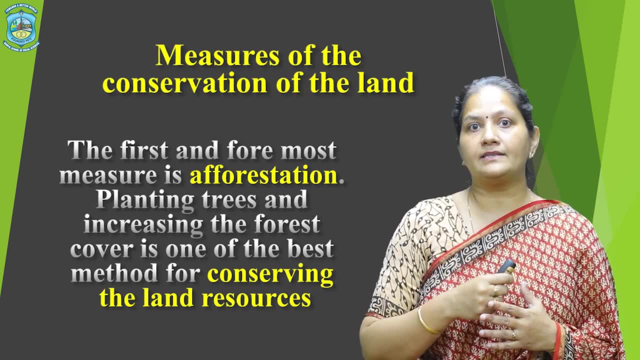 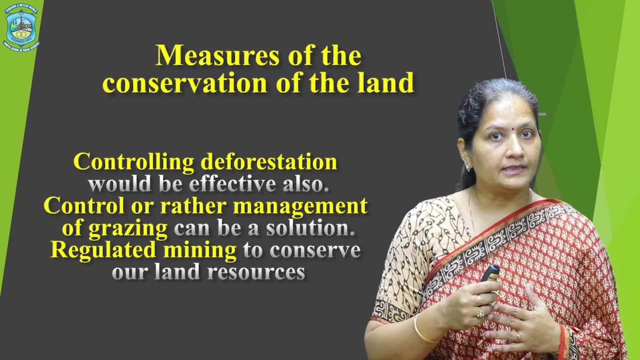 of the land. The first and foremost measure is afforestation. Planting trees and increasing the forest cover is one of the best methods for conserving the land resources And, at the same time, controlling deforestation would be effective also. We all know that overgrazing 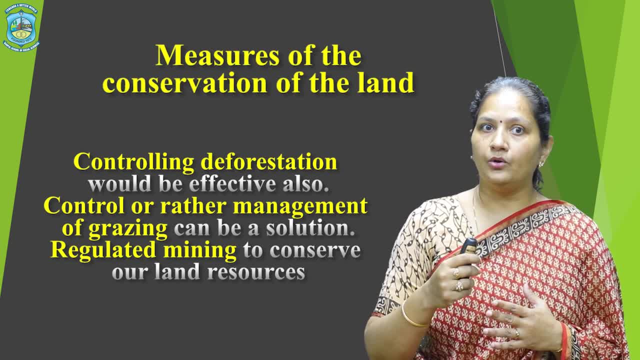 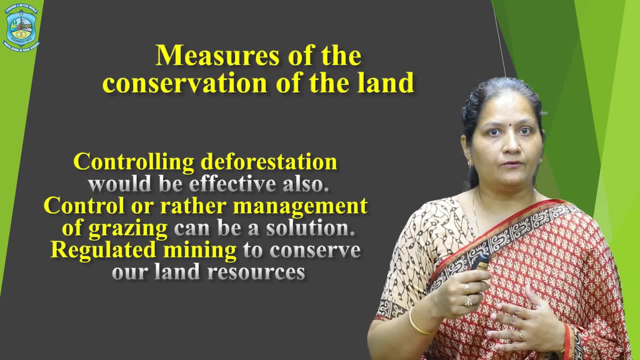 is also increasing the rate of land degradation. So control, or rather management of grazing can be a solution. We human beings do mining for developmental reasons. We cannot stop the mining, But as shortly we might as well build our immediate sa glacial operations, Instead of simply conquering thewhelm of our natural Judeo Mandistum omnidre smartphone. 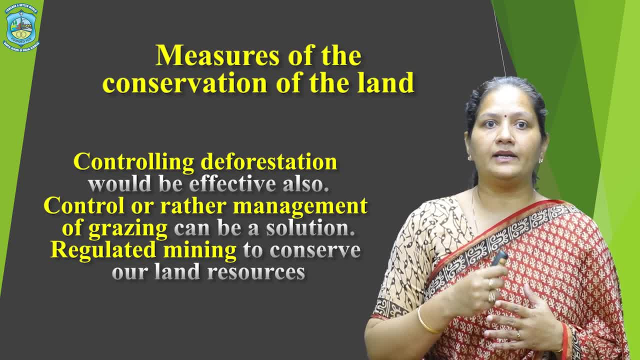 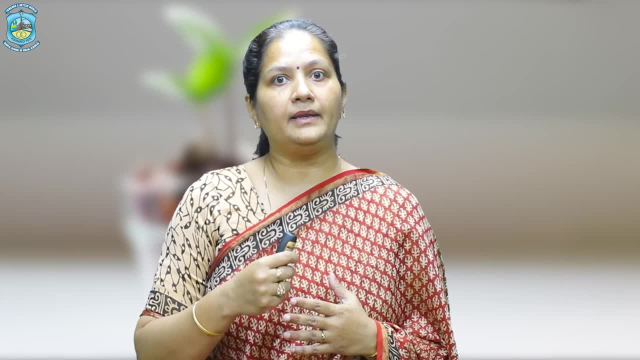 Harvest layer goods. we dry out the product and nourish the soil slightly, change its comfort and vindicate the soil dabei darumu tariz시 harina. income am correlation of the domestic, But we can regulate mining to conserve our land resources. In our agriculture practices we can make specific changes to conserve the land in a plant way. 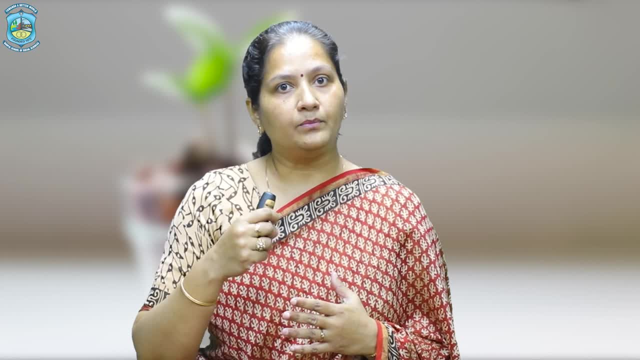 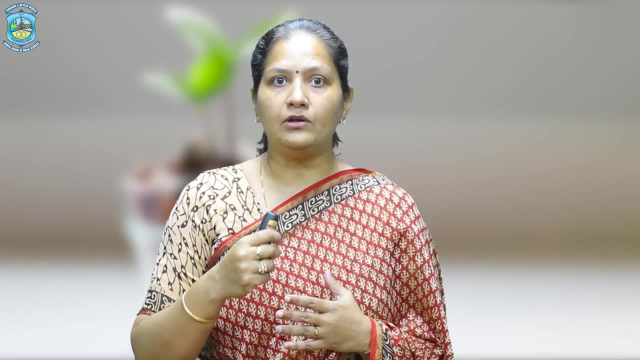 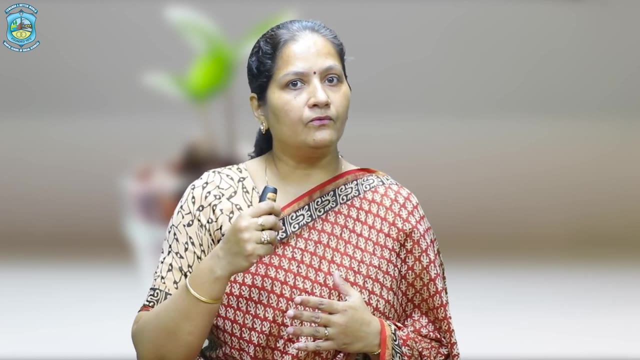 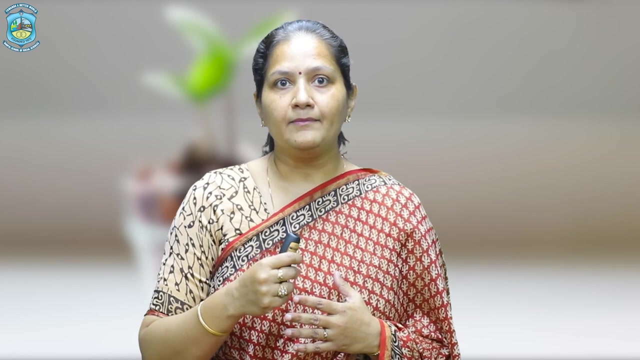 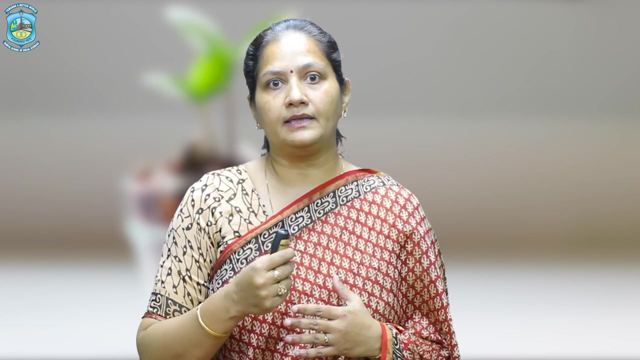 Crop rotation, mixed cropping and plantation cropping can be adapted in agriculture. Plantation of shelter belt is also an effective measure in the conservation of land. Proper and effective management of waste land is also an effective measure for conserving land resources. And I must say planned urbanization, or we can say development of smart cities, can also contribute in the conservation of land and its resources. 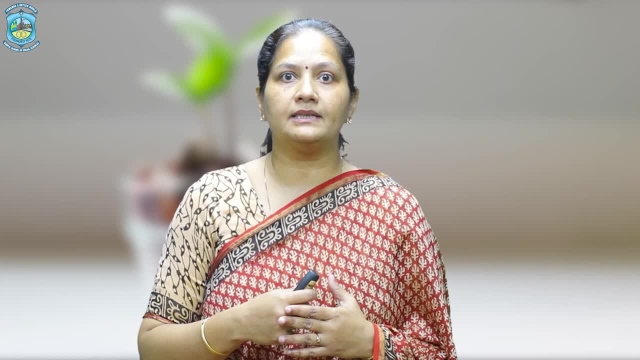 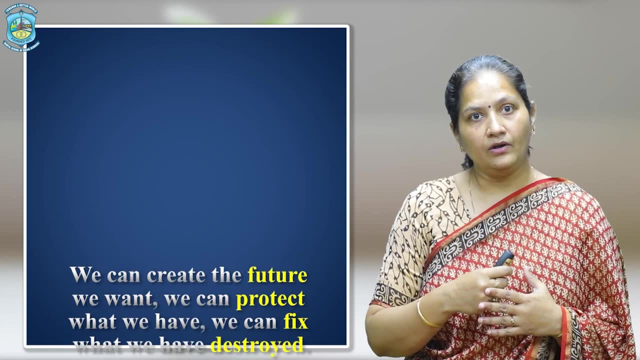 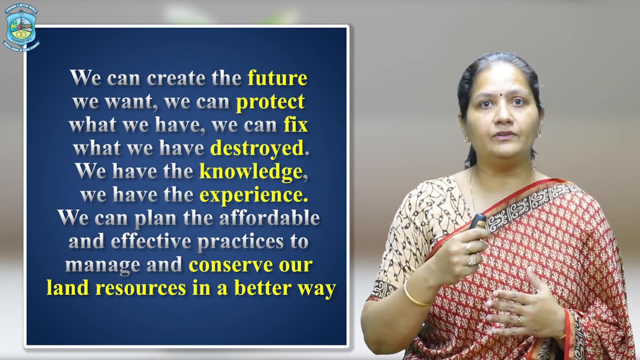 Dear students, fortunately we have resources gifted by nature. By conserving these resources, we can create a better future for our country. We can create the future we want. We can protect what we have. We can fix what we have destroyed. We have the knowledge. 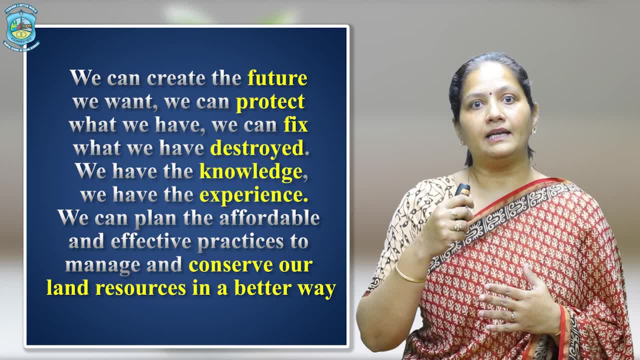 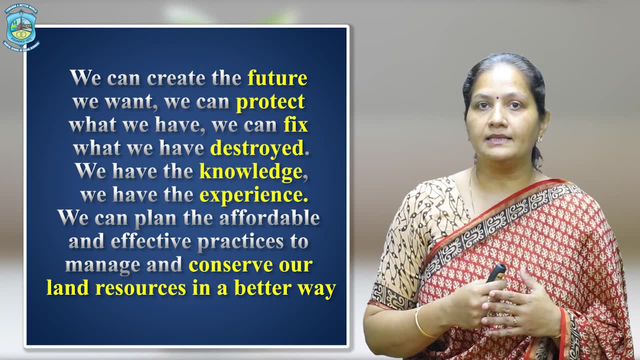 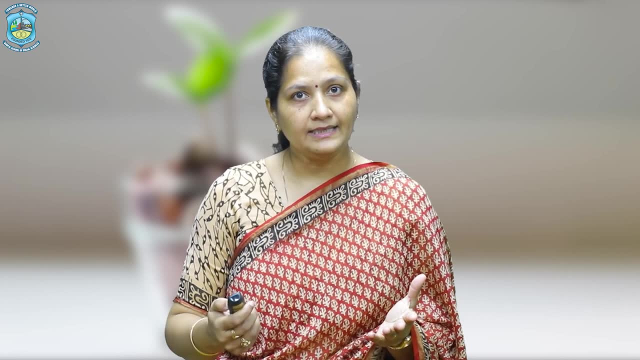 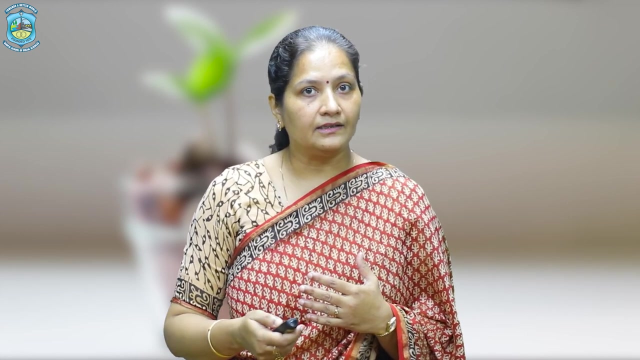 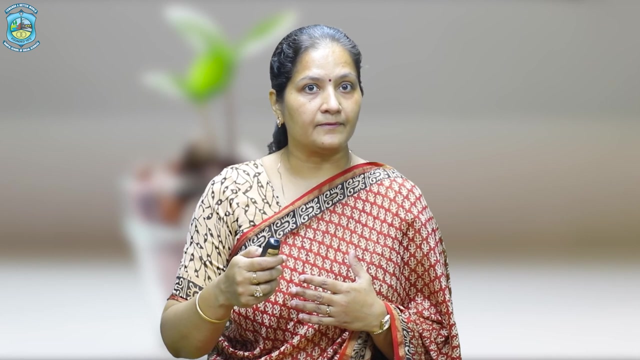 We have the experience, We can plan the affordable and effective practices to manage and conserve our land resources in a better way. It is the way we can ensure food security for us and for our future generations. Let us be proactive: Do protect and conserve our land resources for sustenance of life and for a sustainable future.